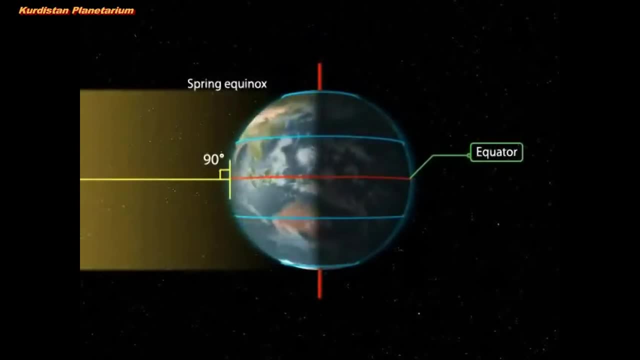 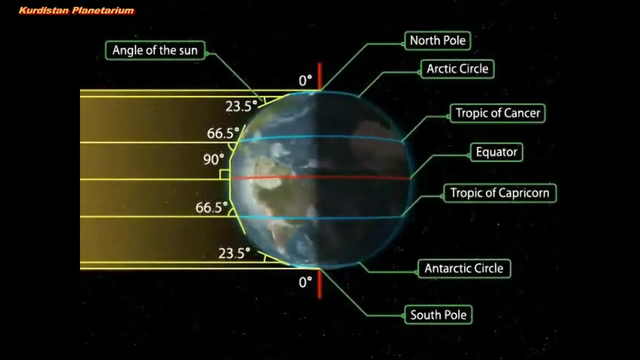 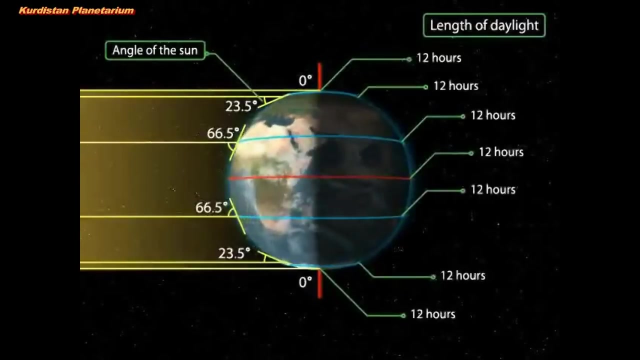 The northern hemisphere is in the Spring Equinox, while the southern hemisphere is in the Autumn Equinox. The angle of the Sun decreases towards the poles. On this day, the two hemispheres receive a similar amount of solar radiation, and the length of day and night is the same at all places on the Earth. 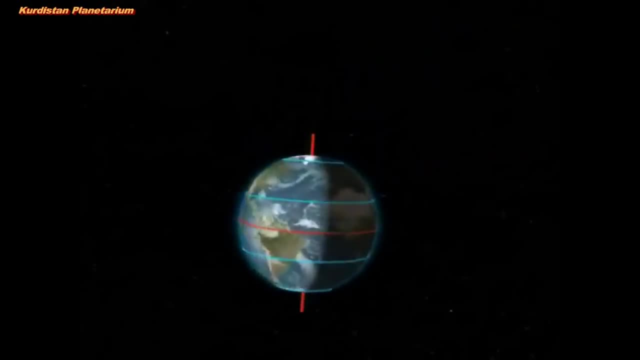 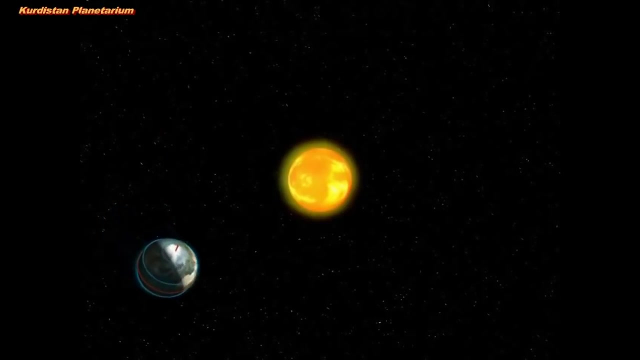 The day and night is the same at all places on the Earth. After this day, it is spring in the northern hemisphere, where the day is longer than the night. In the southern hemisphere it becomes autumn when the day is shorter than the night. 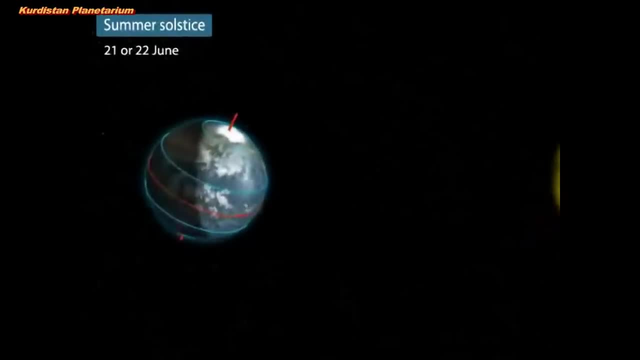 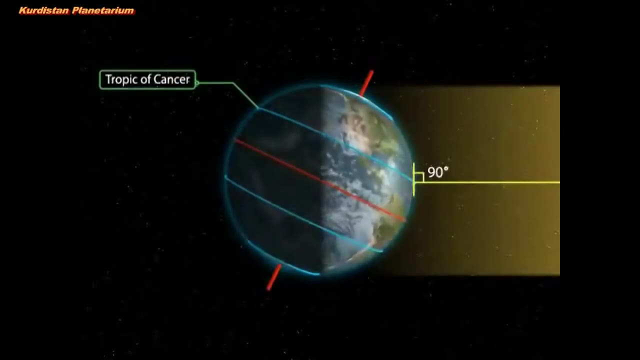 Summer Solstice. On the 21st or 22nd of June, the overhead Sun is over the Tropic of Cancer. It receives It receives the largest amount of solar radiation. At this time the northern hemisphere is in the summer solstice. 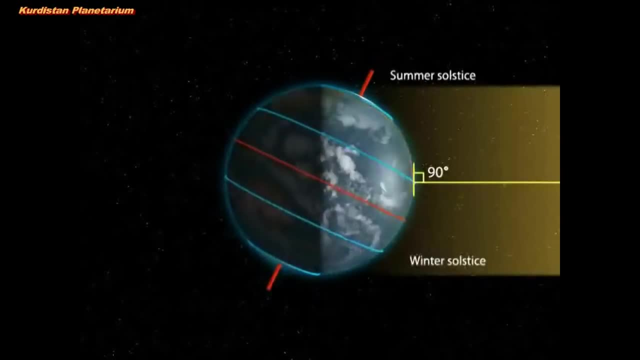 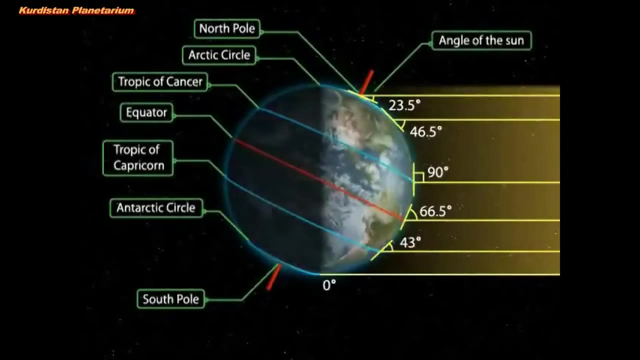 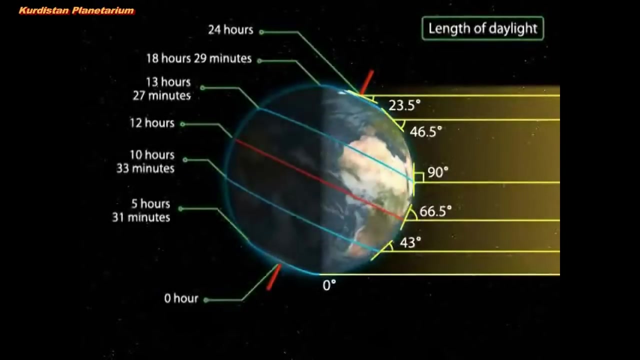 while the southern hemisphere is in the winter solstice, The angle of the sun decreases towards the poles. On this day, the length of daytime of the northern hemisphere is the longest in the year, while that of the southern hemisphere is the shortest in the year. 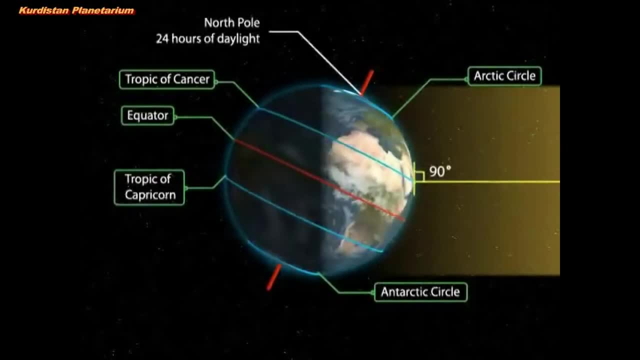 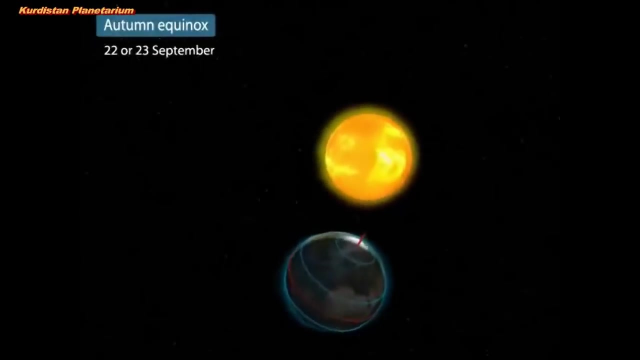 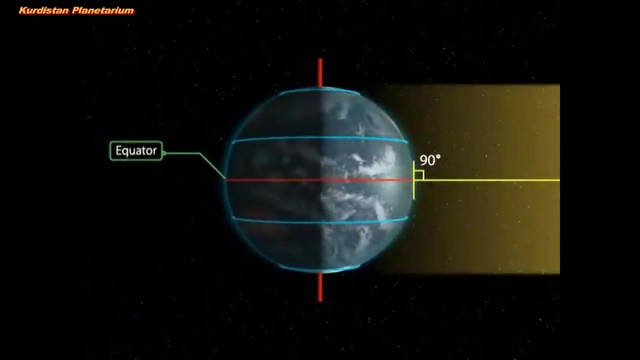 Besides, there are 24 hours of daylight at the Arctic Circle and 24 hours of darkness at the Antarctic Circle. On the 22nd or 23rd of September, the overhead sun is over the equator. again, The equator receives the largest amount of solar radiation. 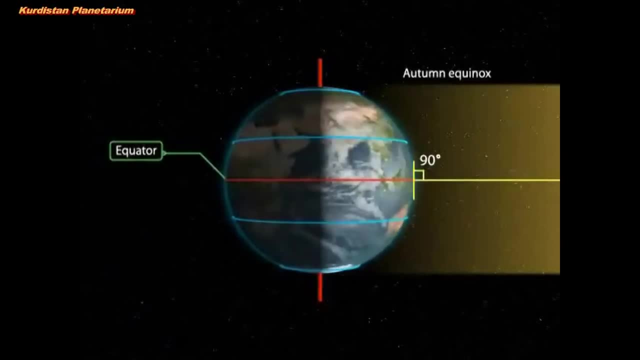 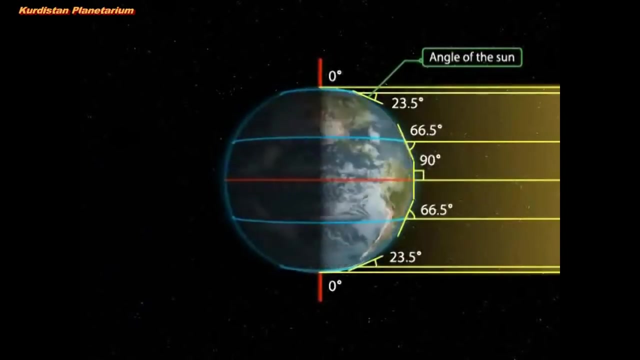 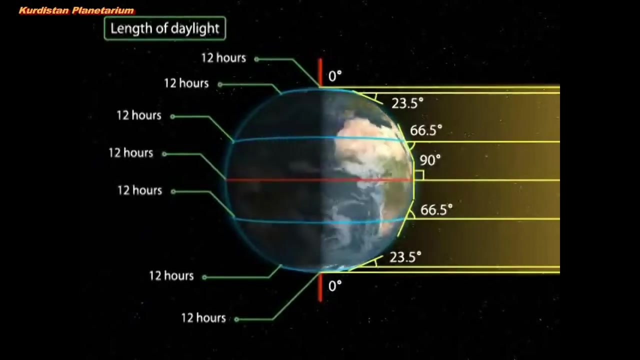 On this day, the northern hemisphere is in the autumn equinox, while the southern hemisphere is in the spring equinox. The angle of the sun decreases towards the poles. On this day, the two hemispheres receive a similar amount of solar radiation.